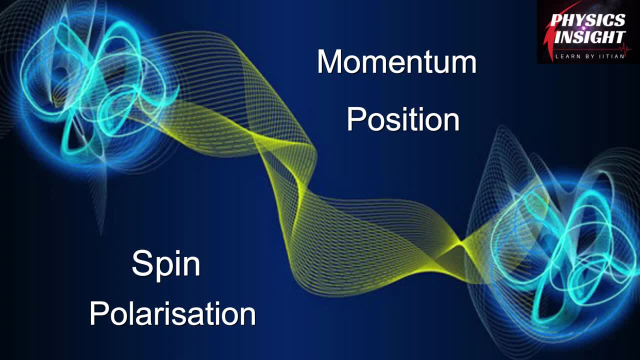 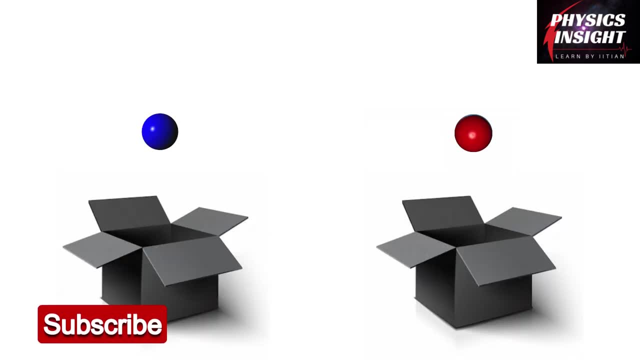 and polarization of one particle, we can predict the measurement of the other particle. Let's take an example. Suppose if we have two balls, one blue and one red, and if we keep them in two boxes and shuffle the boxes after shuffling, we don't know which box contains which colored ball. 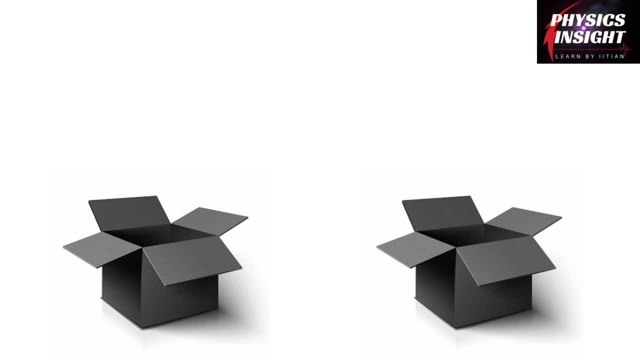 So let's take out a ball from one box and suppose it comes out to be blue. Now, knowing that this, This one, is blue, without seeing the other box, we can say that it contains a red ball. This thing is same as quantum entanglement: that knowing about one state, we can predict. 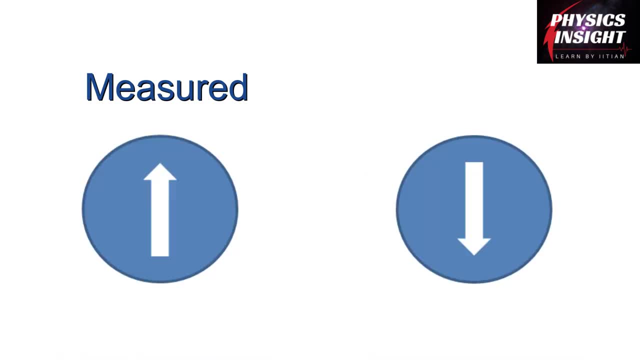 the others. Let's see the same kind of thing in the quantum world. If we have entangled pair of particles such that their total spin is known to be zero, which means these two particles have spin in opposite direction, say z and minus z axis. 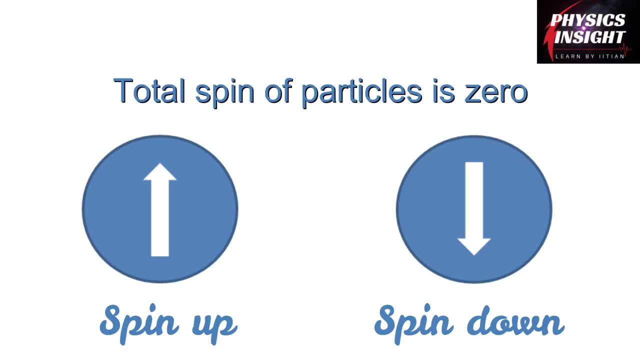 And when we measure spin of one particle, we can predict the spin of other particle at the same instant, While predicting it doesn't matter. that what is the distance between the two particles Sounds weird. Think, if we separate these two particles by few light years, and these two particles are. 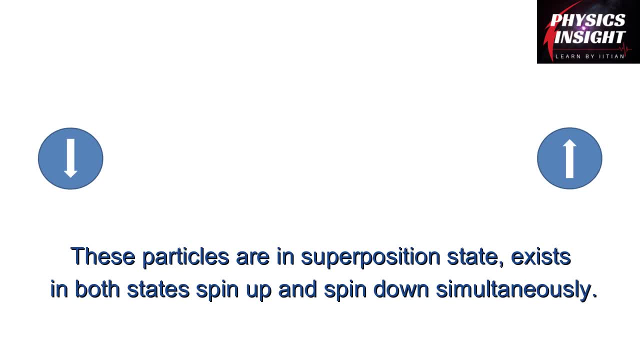 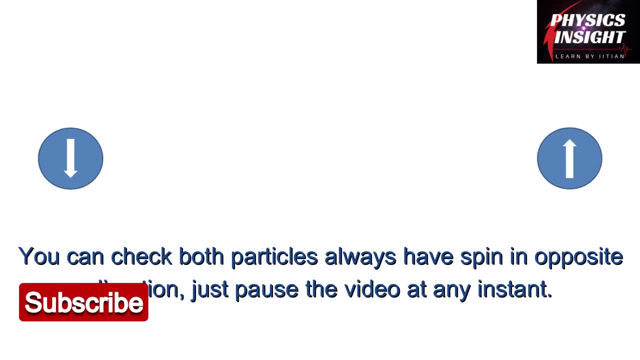 entangled. Now before measurement we can't say which one is spin up and which one is spin down, And also both particles cannot have same spin. As these two particles are entangled, by measuring the spin of one particle we can predict the spin of other particle. 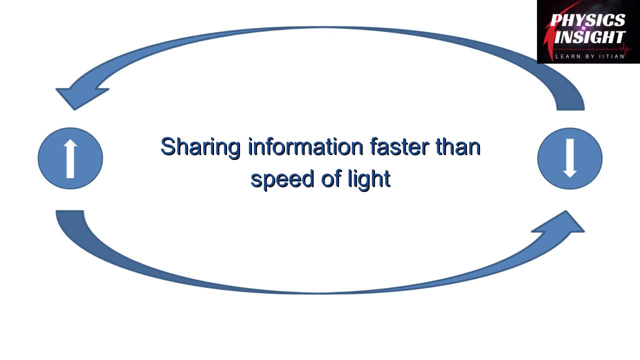 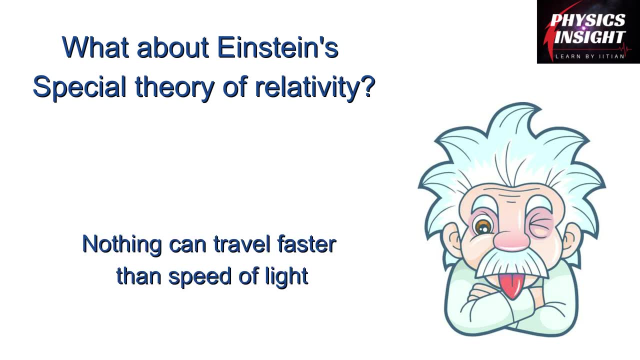 We can say that These two particles are sharing information faster than the speed of light, which violates the Einstein special theory of relativity, which says nothing can travel faster than light. So how these two particles are communicating? This theoretical violation is termed as EPR Paradox. 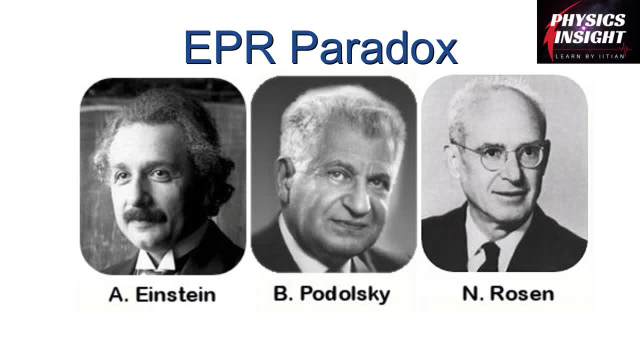 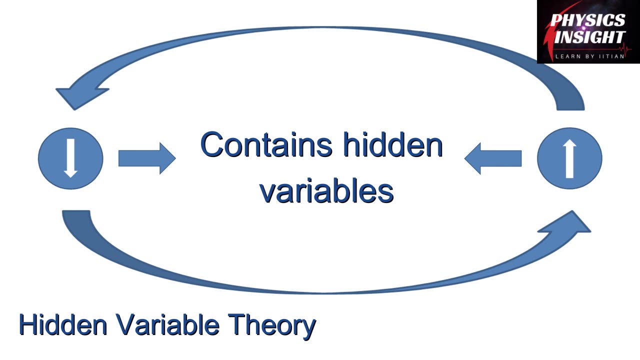 Here EPR stands for Einstein, Podolsky and Rosen. They argued that the description of physical reality provided by quantum mechanics was incomplete and they come up with hidden variable theory, which says that two particles doesn't communicate. They have some hidden variables, or you can say knowledge right from the moment. these particles